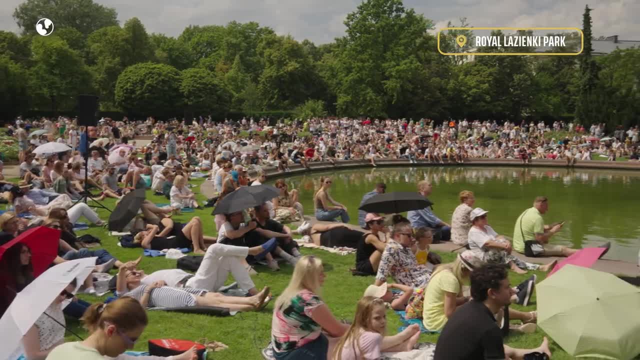 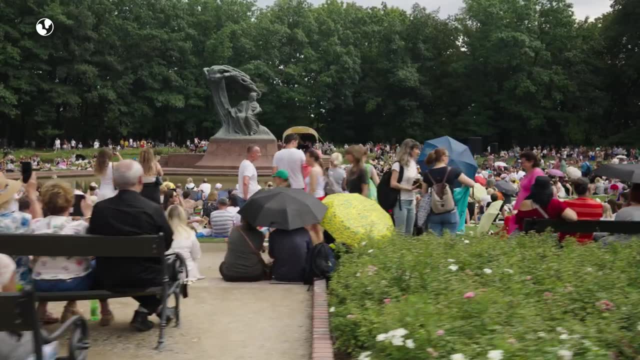 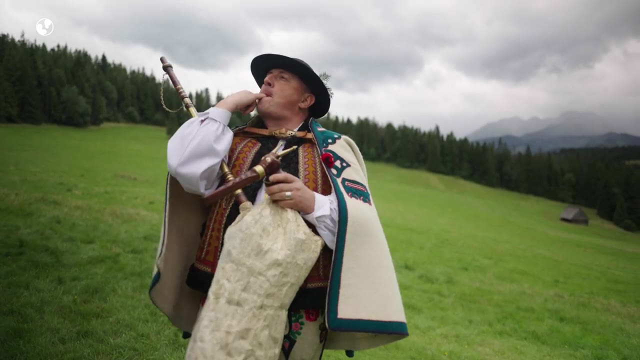 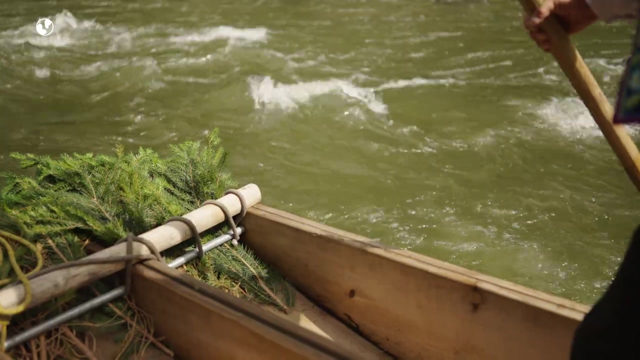 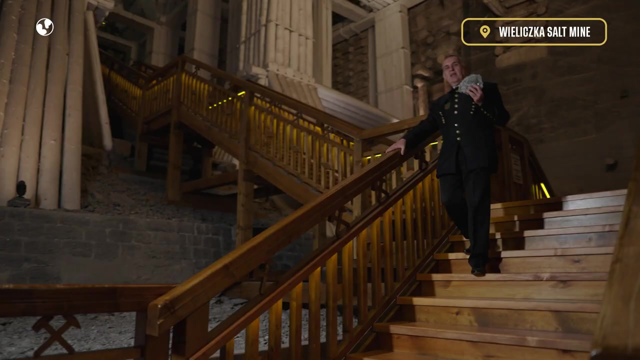 Poland sounds like the music of Chopin. Come and have a listen with me in the park. Poland's love, folklore and tradition- Ha-ha-ha-hey. Poland sounds like a flowing river And, of course, ringing bells. Poland tastes like the salt from Wieliczka mine. 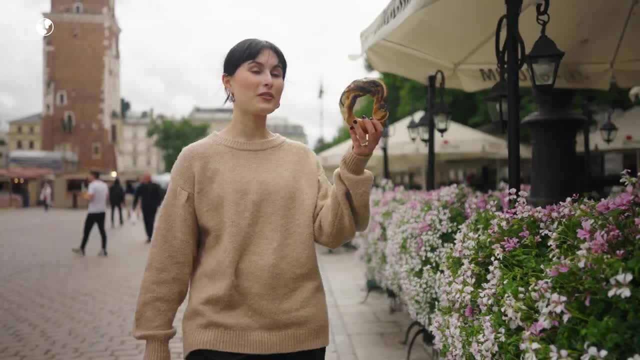 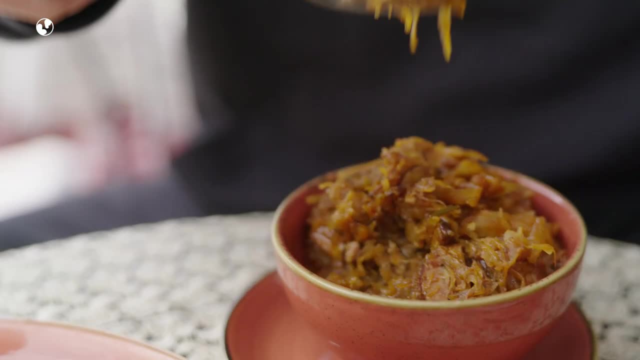 When you're in Kraków, you must try an obwarzenek. The more poppy seeds the better. Have you ever tried this? It's called bigos and it's a delicious cabbage stew. If you want to get the taste of Poland, you have to try our wines. 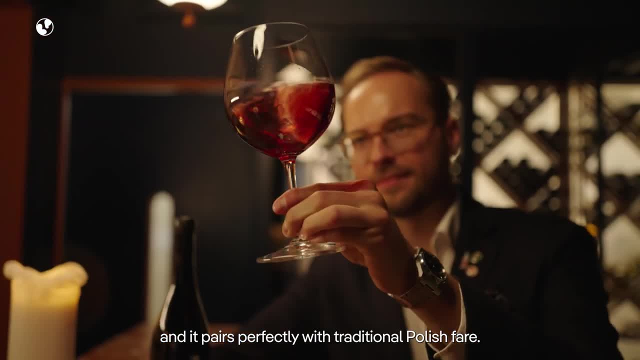 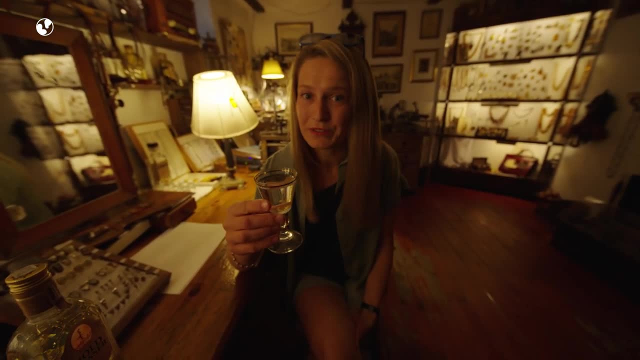 This one grows along Wisła River and it pairs perfectly with traditional Polish fare. One thing you need to try in Gdańsk is goldwasser- Liquor with real flakes of gold in it. Beer with raspberry syrup is a summertime specialty. 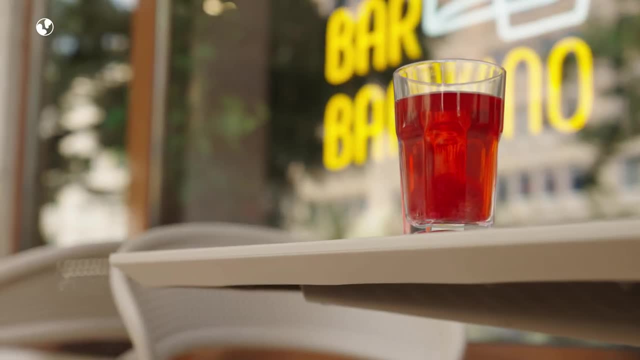 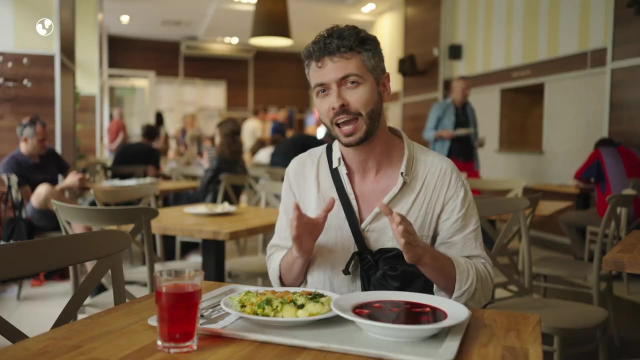 For something more refreshing, try kompot, A classic beverage made from synerg fruits, A holdover of the Soviet Union. Milk bars are the uniquely Eastern European style of cafeteria-restaurant hybrid, where you can get cheap homestyle meals like barsz or schabowy. 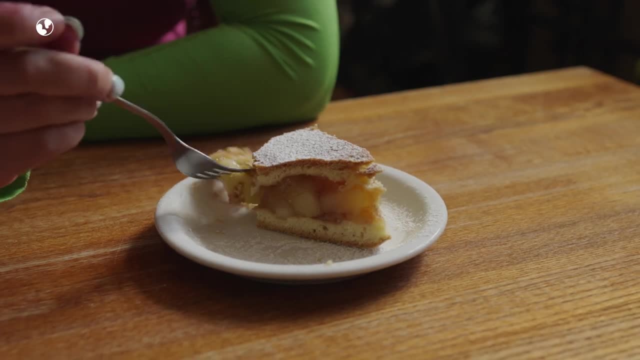 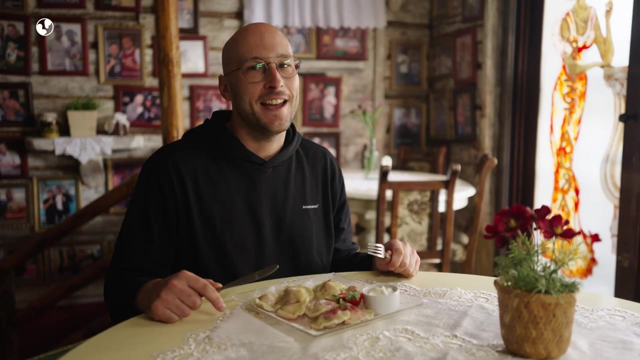 There are many great desserts in Poland, but nothing beats szalotka in a mountain hut. Whatever the case, you can't go wrong with jelly-filled pączki. And of course, everybody loves pierogi. Did you know that you can even have them for dessert with fruit filling? 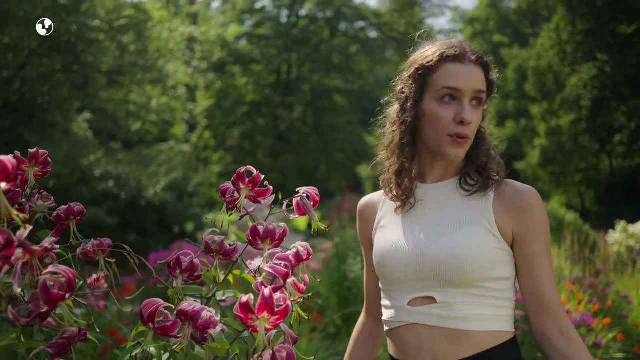 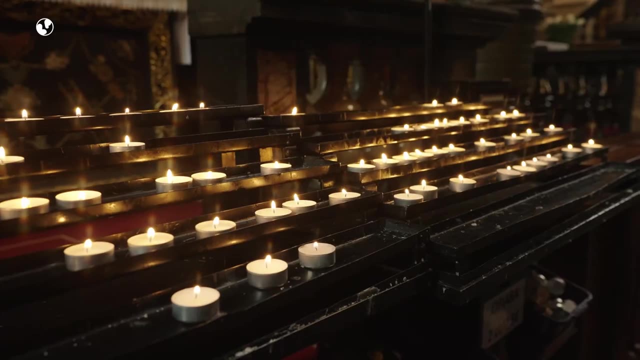 Do you smell that? It's the smell of flowers. in the royal gardens of Łazienki Park In St Mary's Basilica, incense fills the air. Poland smells like wild mushrooms. Picking them could be our national sport. 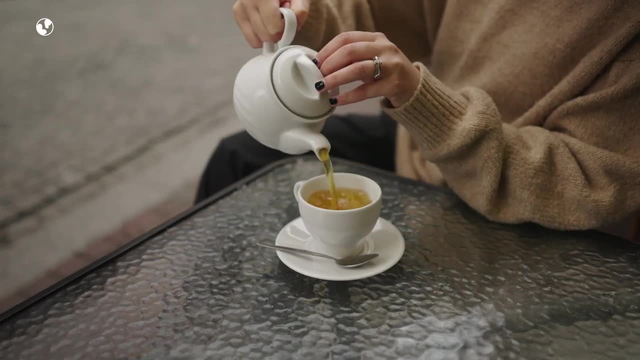 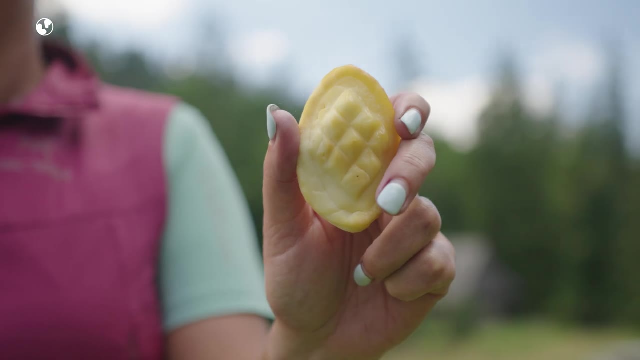 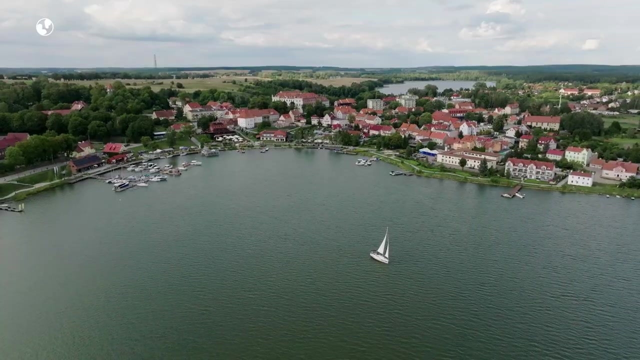 Poland smells like fresh brew tea in a charming alleyway. Poland smells like a bonfire with friends. Poland smells like a smoked cheese from a batówka. You can find these smokehouses all over the south of Poland. What does Poland feel like? Poland feels like the wind in your sails.